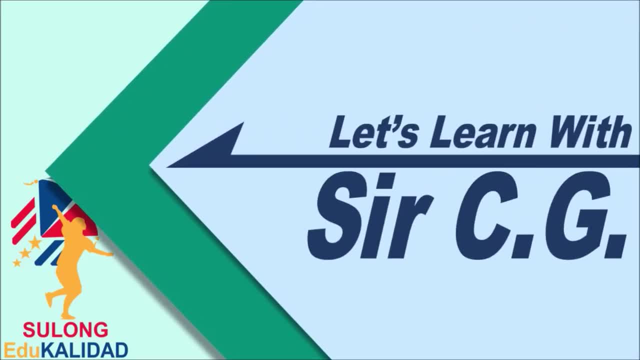 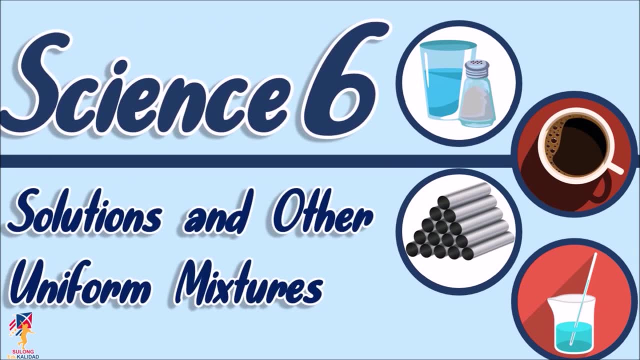 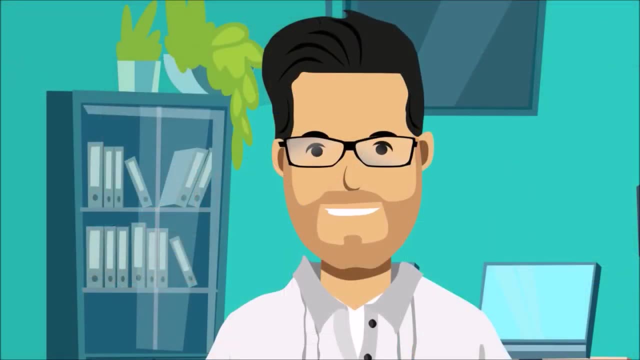 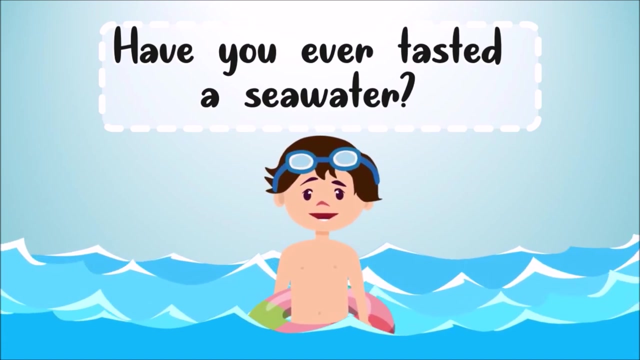 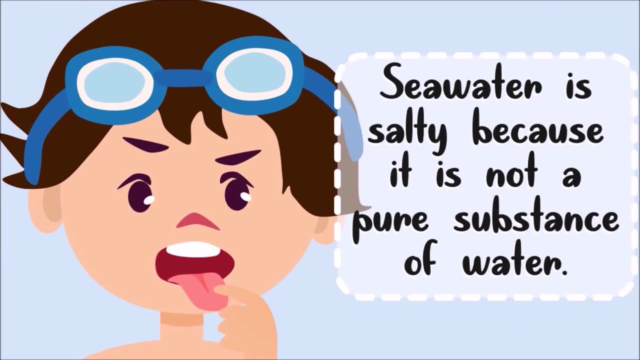 Hi there, my name is Teddy and welcome to science. Let me ask you a question: Have you ever tasted a seawater? What does it taste? It's salty, right? That is because seawater is not just a pure substance of water, but it is a mixture. If you put some seawater inside a jar, it 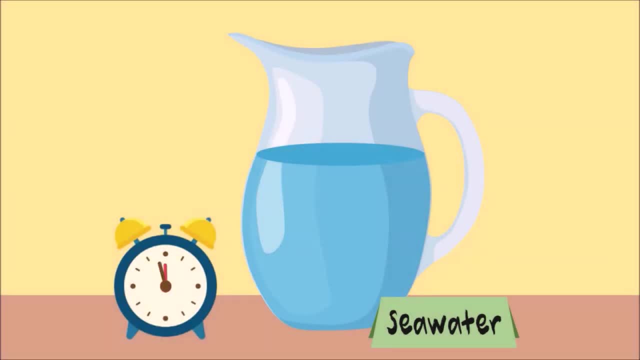 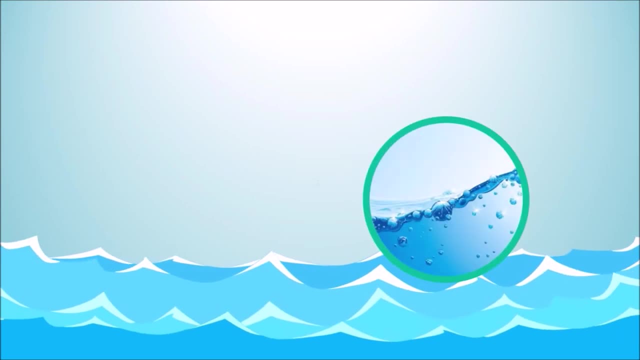 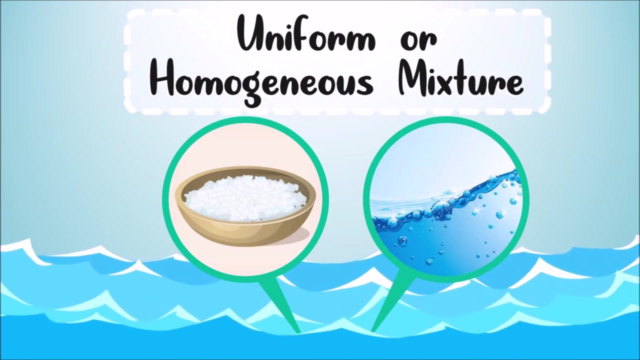 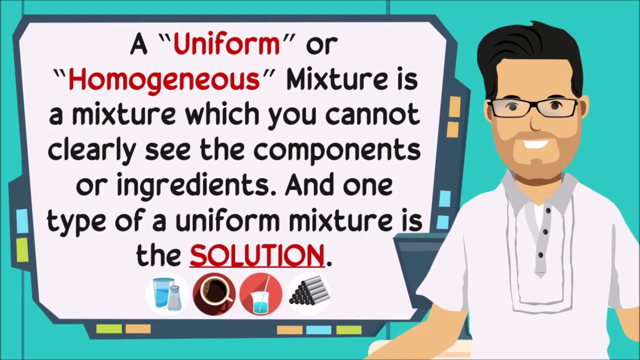 will remain salty no matter how long you let the jar sit. Seawater is a mixture of water and salt And this is a good example of uniform or homogeneous mixture. A homogeneous mixture is a mixture which you cannot clearly see the components or ingredients, And one type of a uniform mixture is the solution. 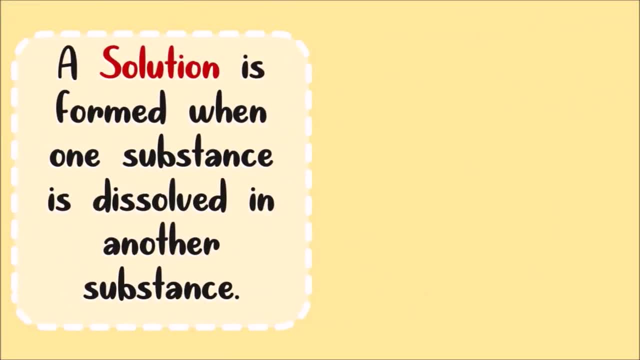 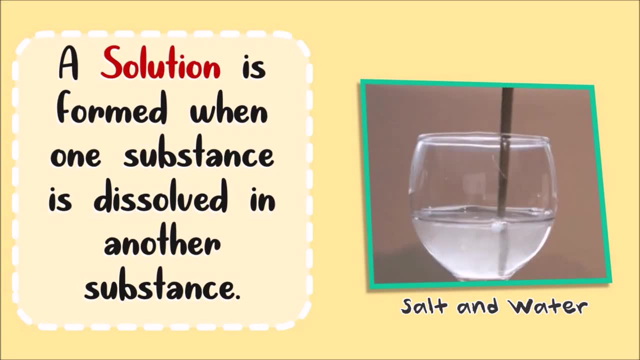 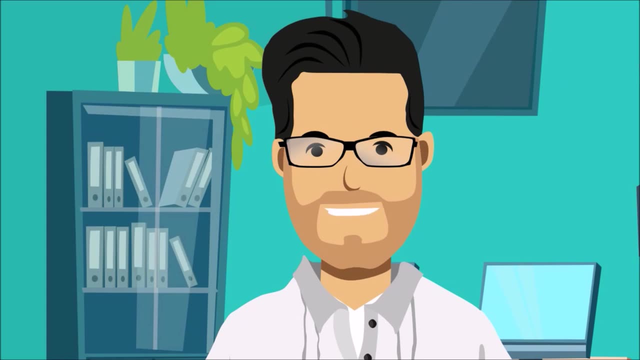 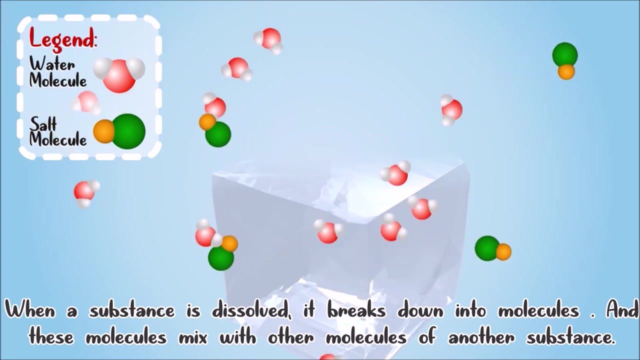 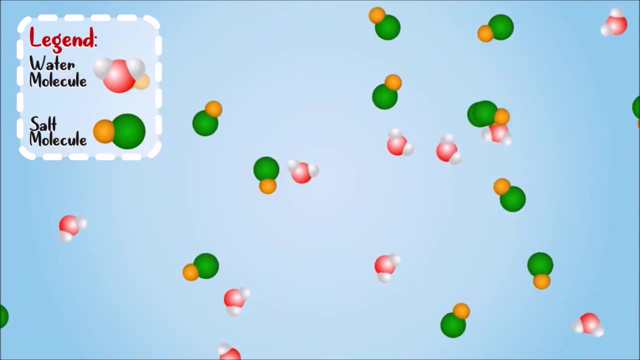 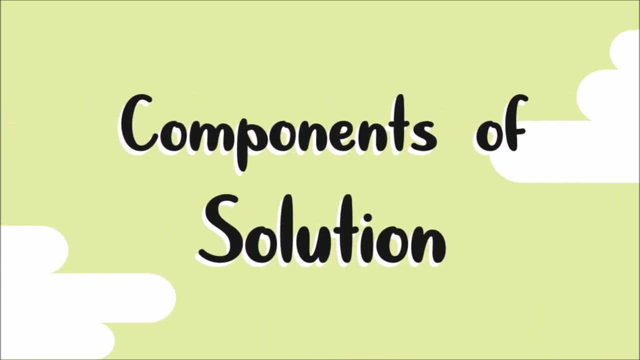 What is solution? A solution is formed when one substance dissolves in another substance. How does it happen? When a substance is dissolved, it breaks down into molecules And these molecules mixed with other molecules of another substance. How does it happen? A solution is formed when a liquid is dissolved in another survés. 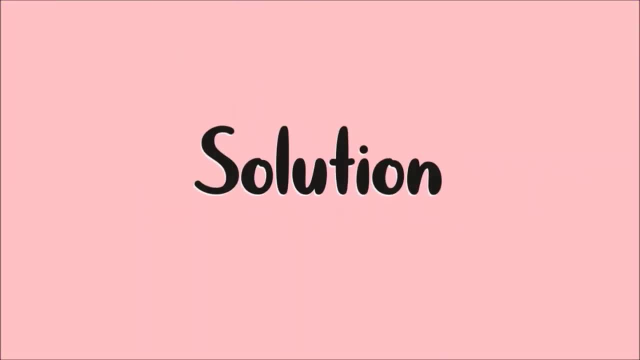 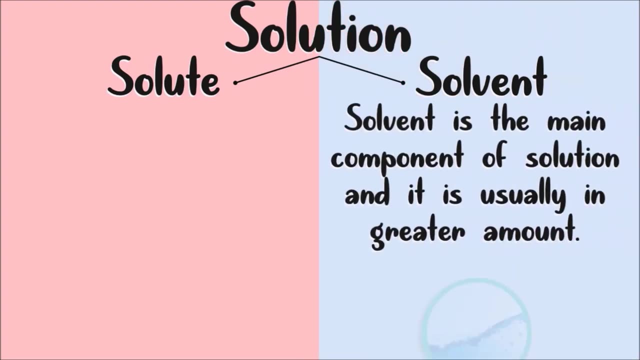 Let me ask you a question. Do we know what the solute means? Solution is played in a system of inhaling and exhaling of another substance. One solution cannot be defined by itself. What is solution? Solution is played with another substance. You see, the solution contains solutes and solvents. Solvents are the main components of solvents and solvents are not the same as the main one. However, two people know what a solvents are, which君 and I'll witness hack at that. Solvents are those high and these solvents contain solvents and solvents. So, for example, when a solution is after dilution due to the quiet cooling systems, after dilution the solvents cause Houlihan's ponejiance. 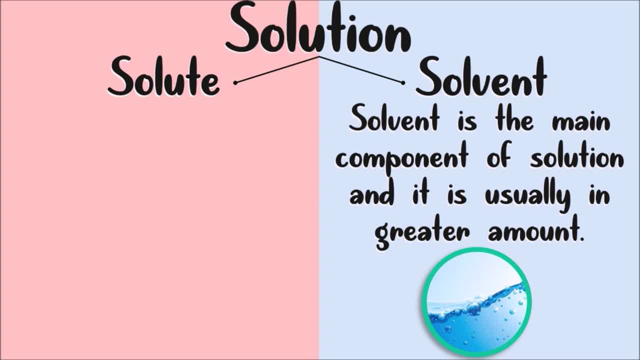 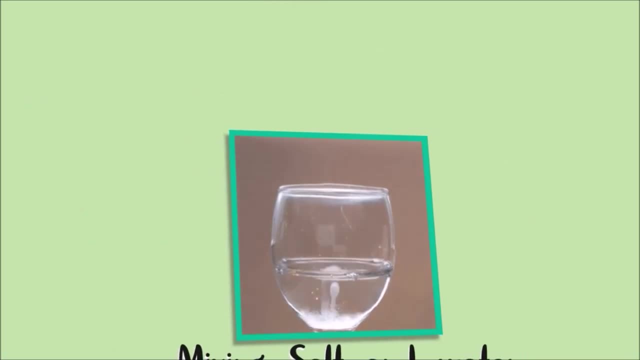 That's my right. It is usually in greater amount. On the other hand, solute is the additive or substance being dissolved in the solvent. Solute is usually lesser than the solvent. For example, in the mixture of salt and water. the salt is dissolved in water. 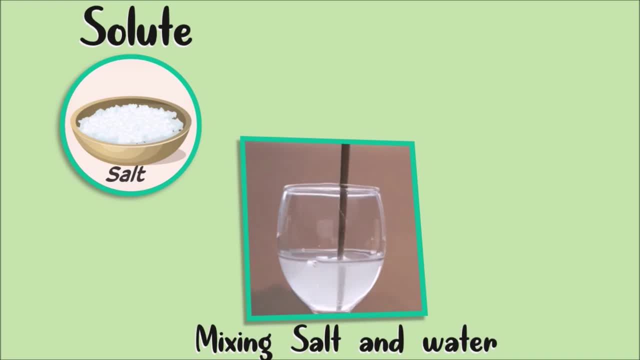 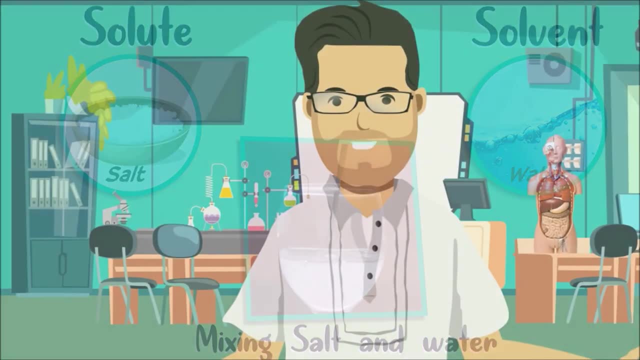 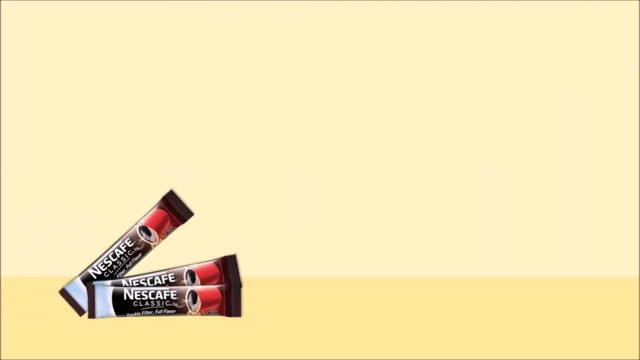 Therefore, salt is the solute and water is the solvent. Another example is when you try to make a coffee First, you need to have a coffee powder, hot water and sugar if you want to make it sweet. Can you identify among these which are the solute and solvent? 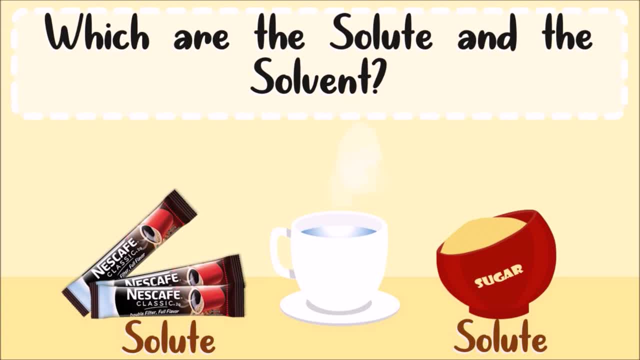 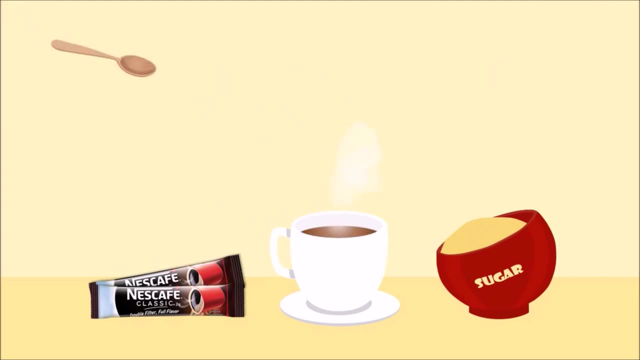 The solute are coffee powder and sugar, And the solvent is hot water. If we mix these together, the coffee powder and sugar will slowly dissolve into the water, And if you mix it using your spoon, you will no longer see any powder of coffee or even a crystal of sugar. 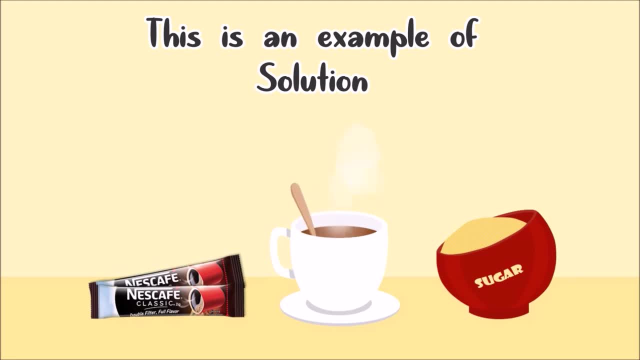 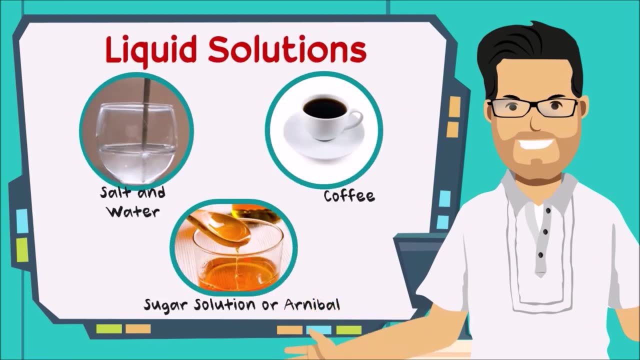 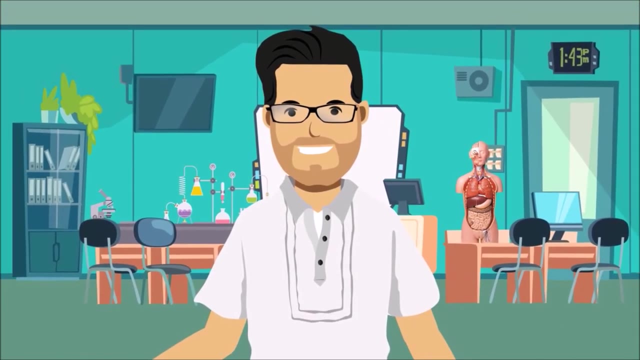 And that is an example. And that is an example of solution. Some examples of solution mixture that I had shown you earlier are liquids, But there are also other type of homogeneous mixtures which are in other phase of matter, such as solid and gas. 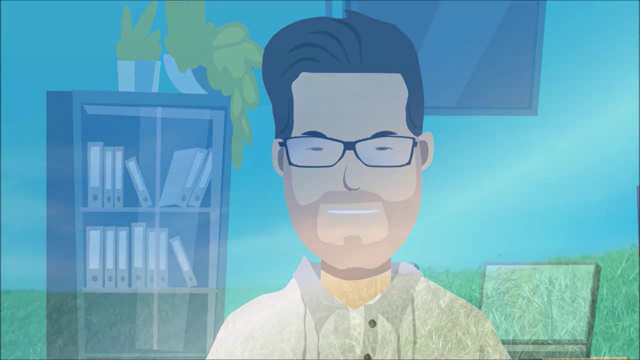 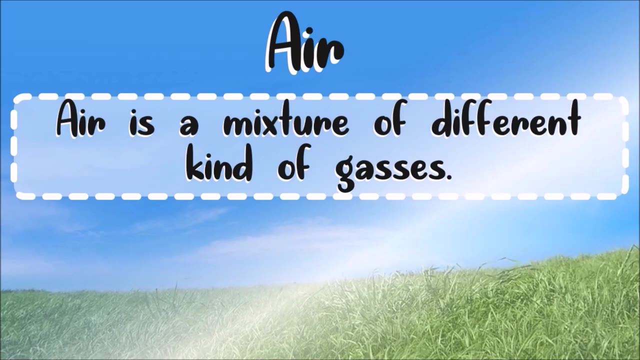 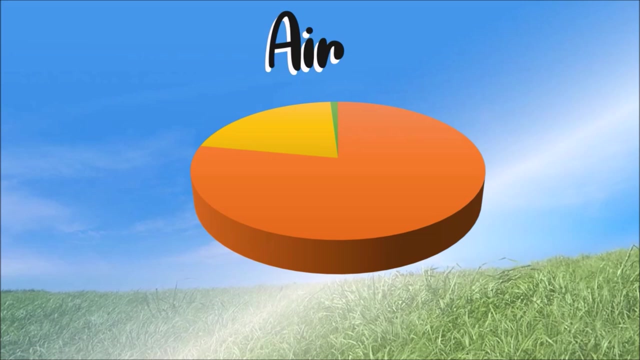 Examples of homogeneous mixture in gaseous form. Examples of homogeneous mixture in gaseous form are air. Air is actually a mixture of different kinds of gasses. According to study, our atmosphere, or the air around us, is composed of 78% nitrogen. 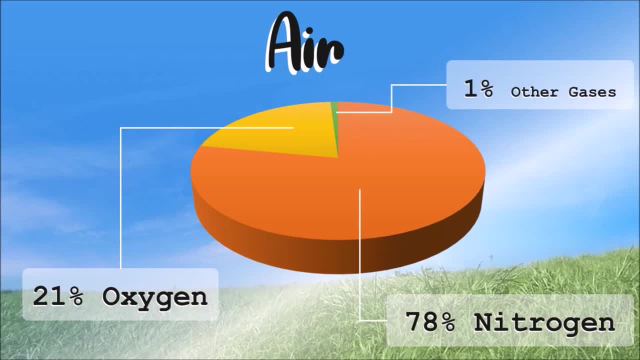 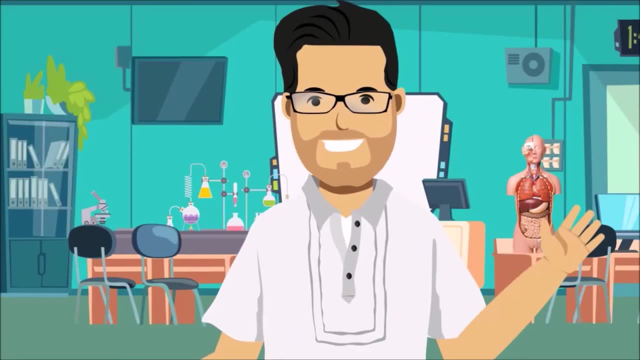 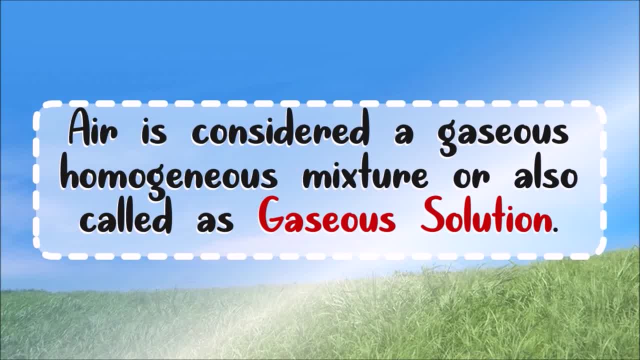 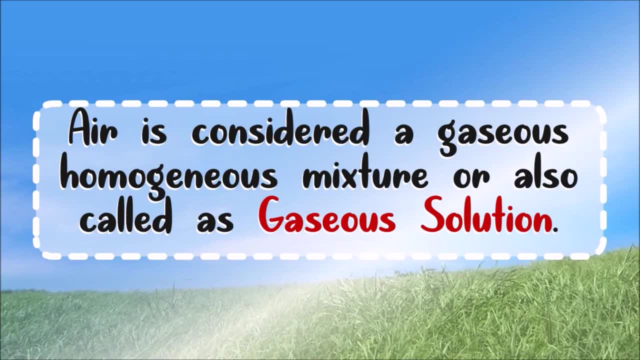 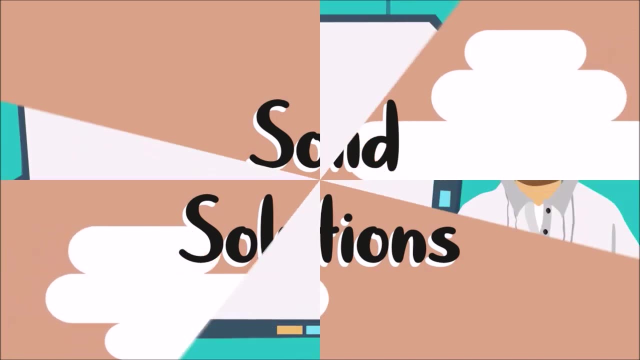 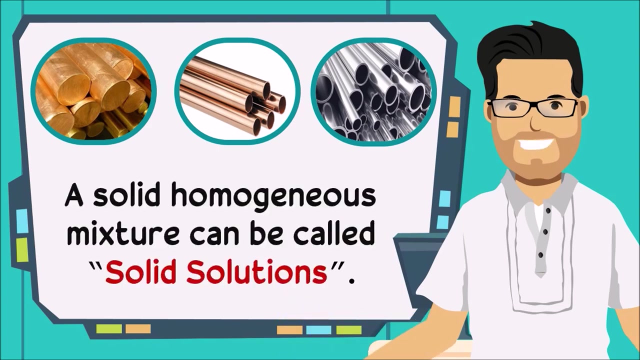 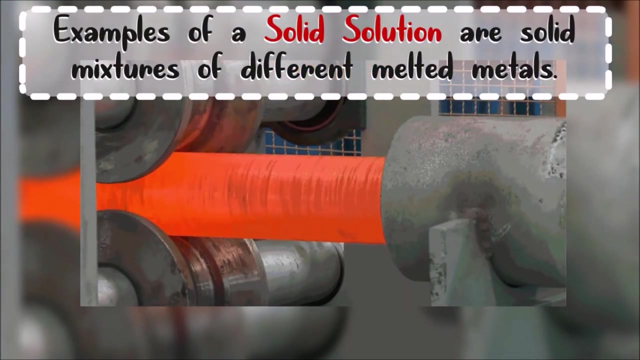 Since we cannot easily separate this from other gasses, different gases from each other, air is considered a gaseous homogeneous mixture or also called as gaseous solution. there are some solutions also in solid form. solid homogeneous mixture can be called solid solutions. examples are solid mixtures of different melted metals. these mixtures of metals are also. 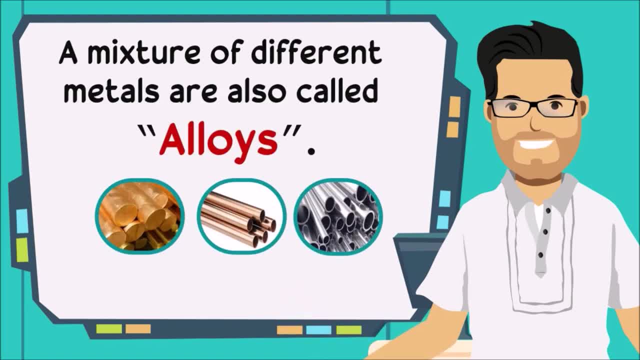 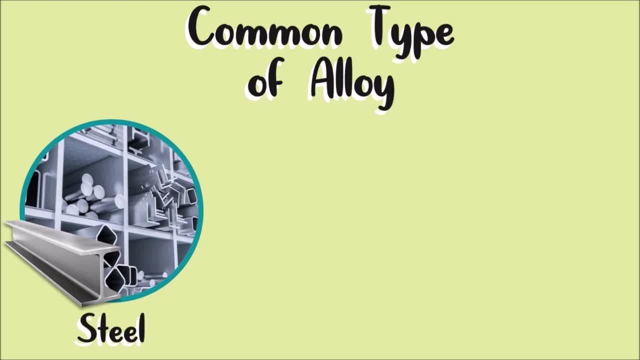 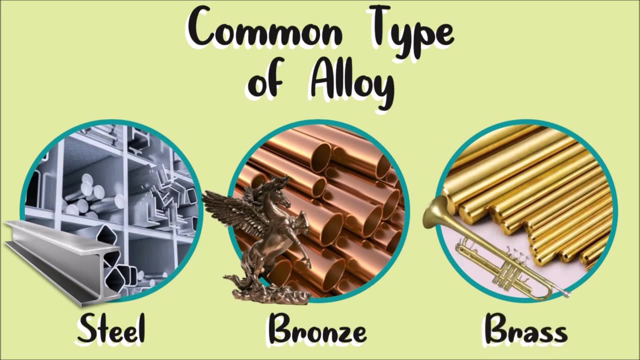 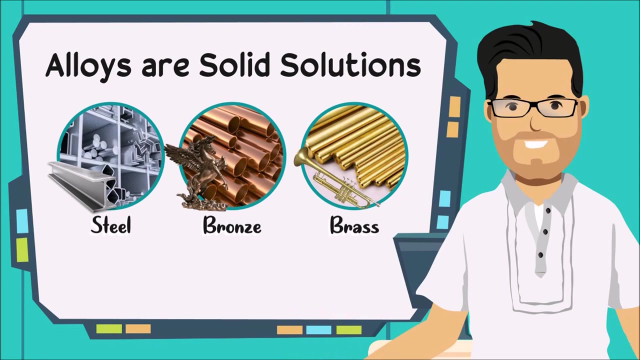 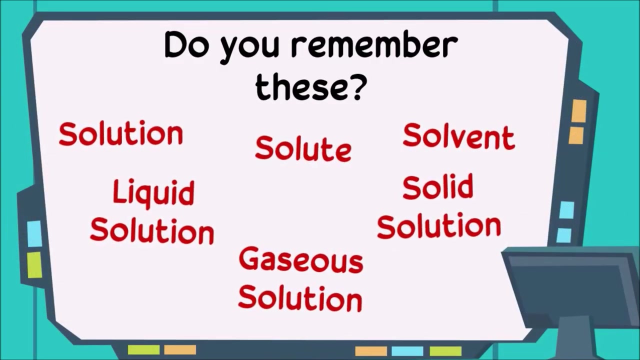 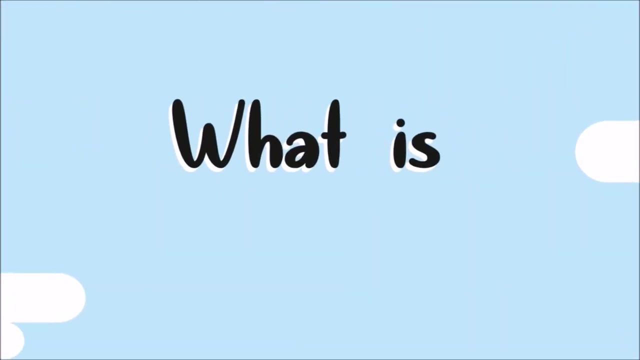 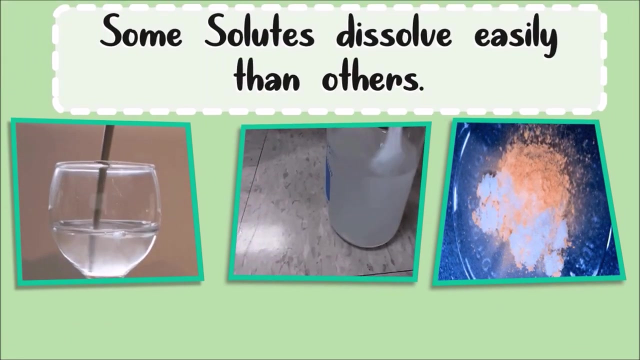 called alloys. we actually see many alloys around us. the most common type of alloy are steel, bronze and brass. remember that these metals are mixed with metals and metals are solid and mixtures. and these are examples of solid solutions. do you remember these? some solutes dissolved easily than others. this property of solute is called. 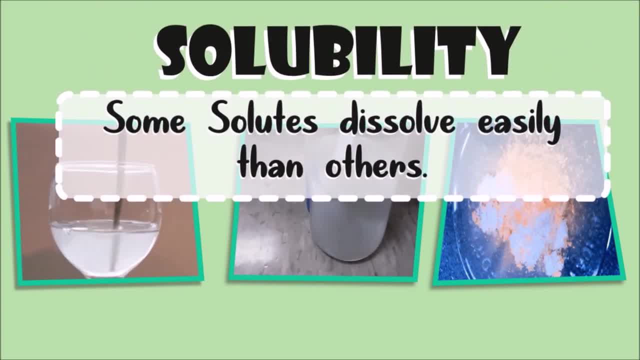 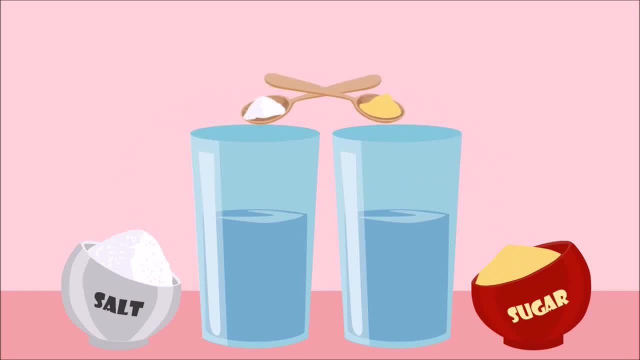 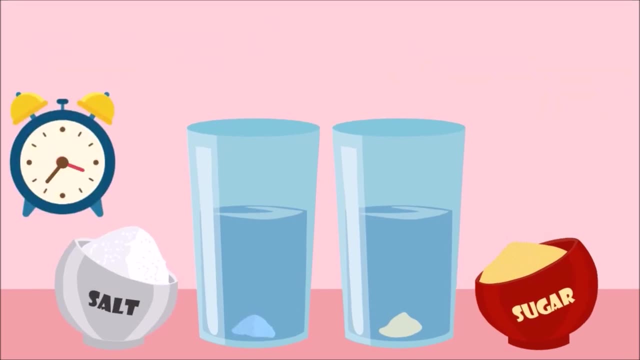 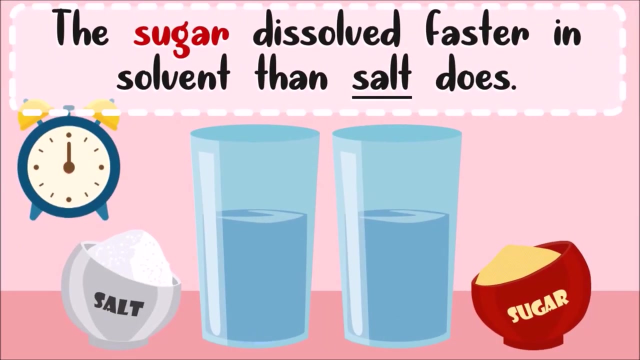 solubility. draw another solution from the Whoever above the image of sufficient skalabai all impairment. functional table plays key. до when you put sugar and salt in separate glasses with the same amount of water, which one do you think will dissolve faster. this sugar dissolved faster in. solvents and salt does. this is because sugar is more possible when found thatopian gale, Panamanian glo Consecutor drink malode approaches to l seja, the descendant from인이 Cal 여러 soleil diлючerya, another power source and number of degrees, ag instruction, life and defense, is present on a. 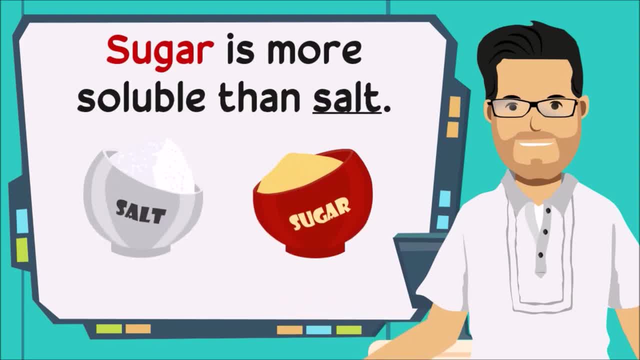 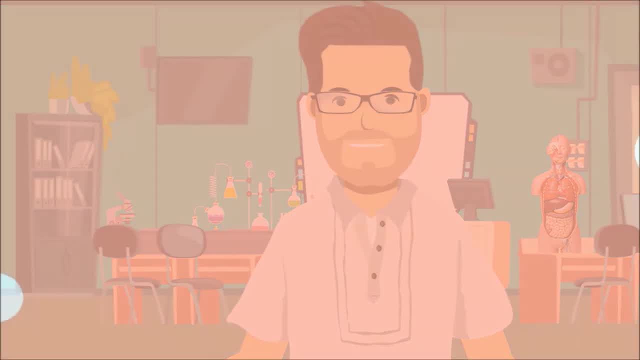 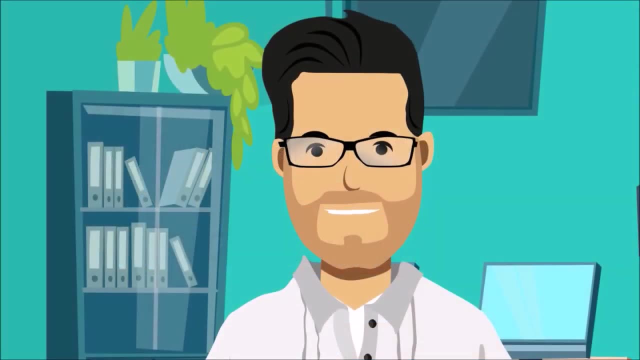 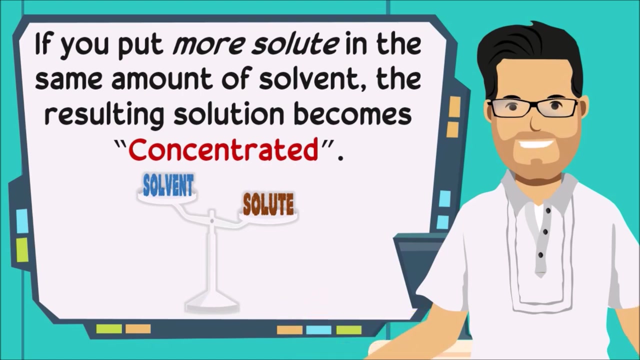 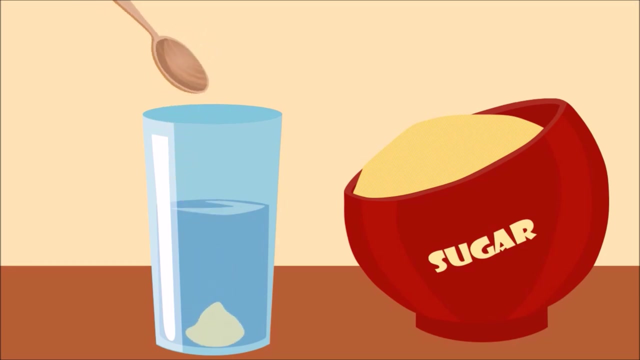 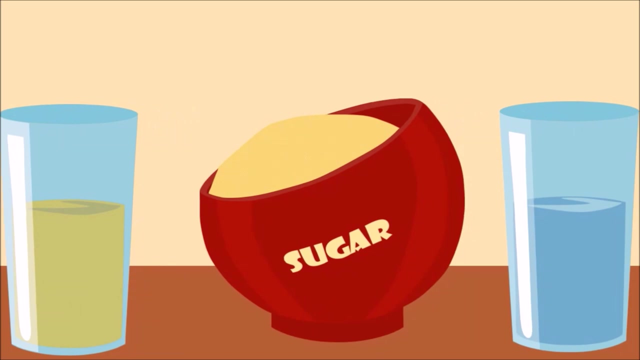 soluble than salt solution also vary in concentration and dilution. what about these? if you put more solute in the same amount of solvent, the resulting solution becomes concentrated. example, if you put so much sugar in a glass of water, these sugar solution becomes concentrated. on the other hand, if you add more solvent, 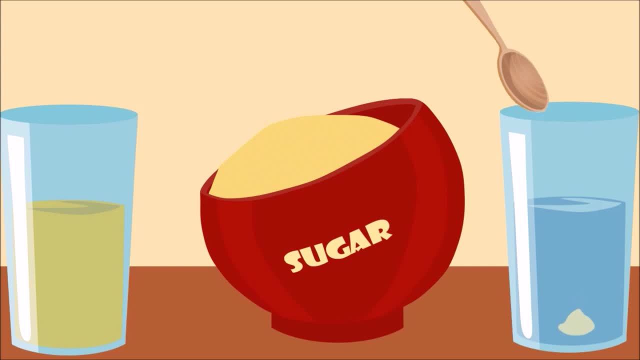 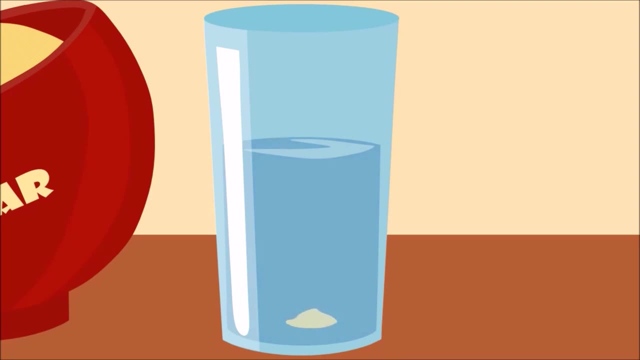 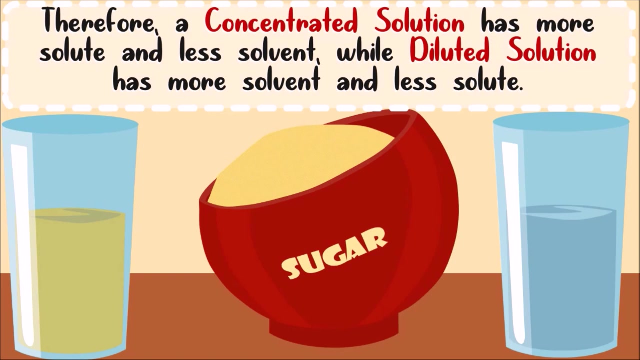 than the amount of salt solution, the resulting solution becomes concentrated. on the other hand, if you add more solvent than the amount of salt solution 6, the resulting solution becomes diluted. therefore, a concentrated solution has more sobre and less solvent, while diluted solution has more solvent than the concentrated one. 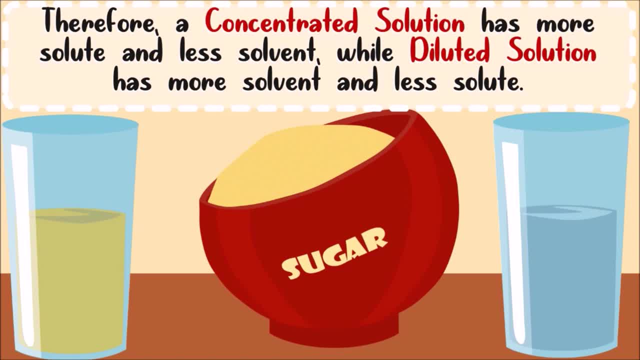 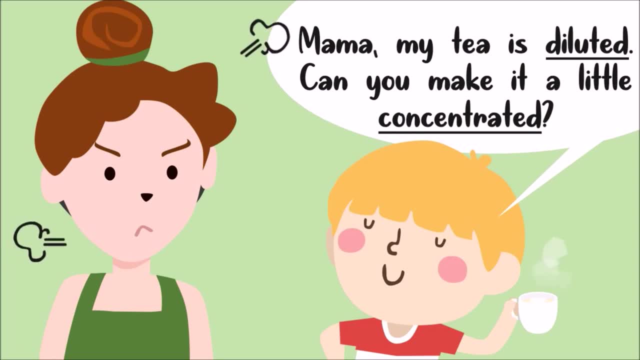 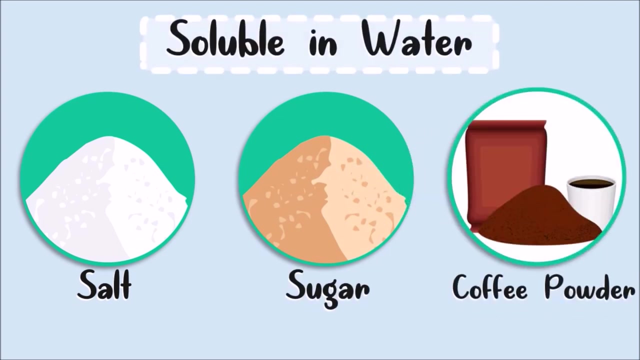 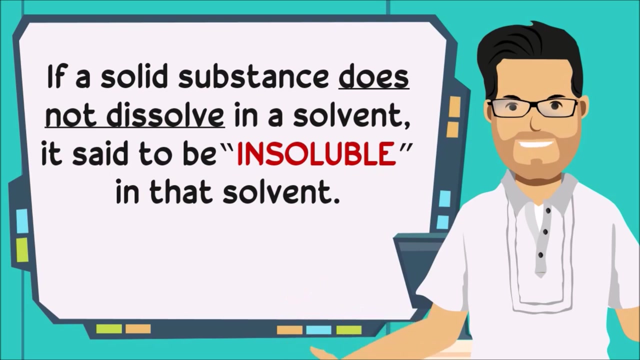 and less solute. That is why, if you want to complain about your tasteless tea, tell your mother that your tea is diluted and you want it a little concentrated. Salt, sugar and coffee powder are solids which are soluble in water. But if a solid substance does not dissolve in a solvent, 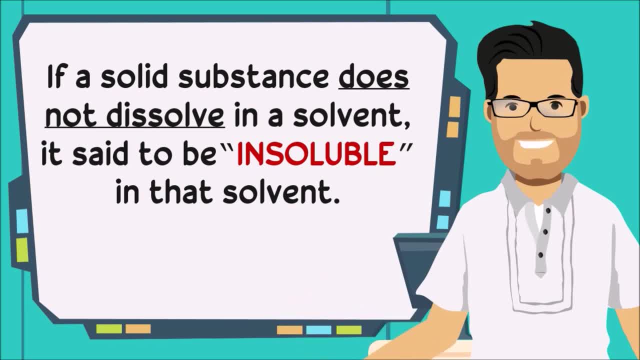 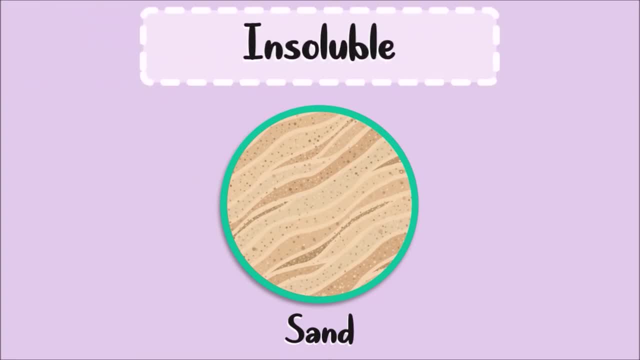 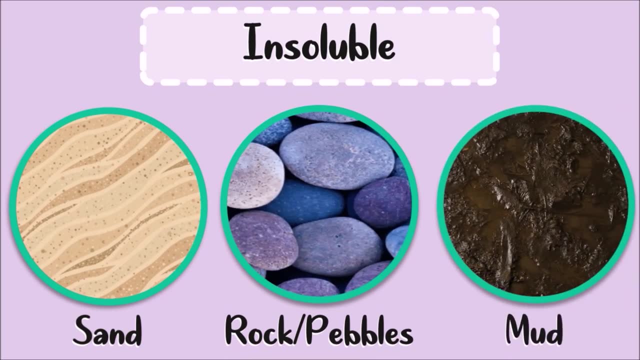 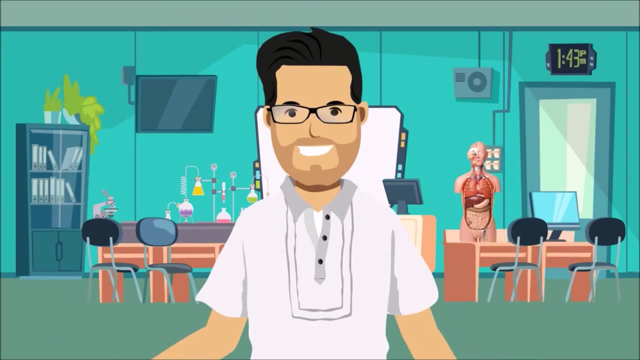 it is said to be insoluble in that solvent. Example of insoluble substance are sand. Sand is insoluble in water. Rocks and mud are also insoluble in water. Salt, sugar and coffee powder are solids, but did you know that there are also liquids? 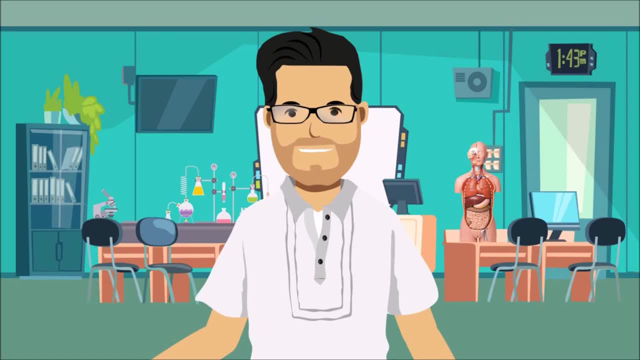 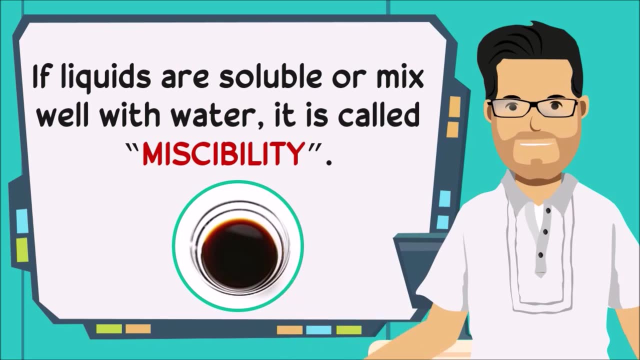 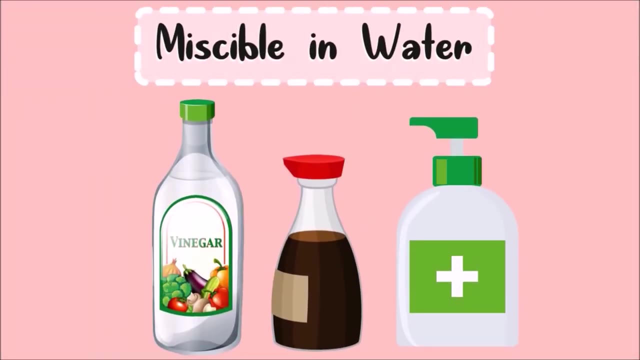 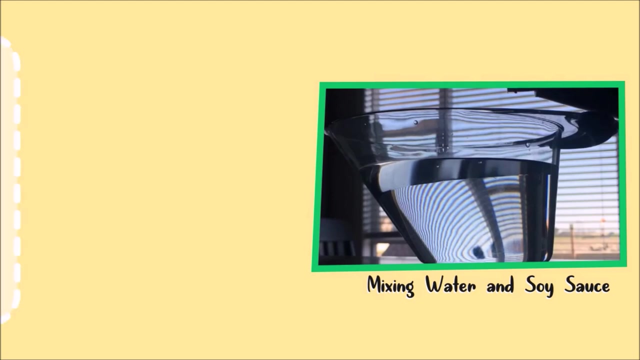 that are soluble in other liquids. That's right. If liquids are soluble or mix well with water, it is called miscibility. Liquids like vinegar, soy sauce and alcohol are miscible in water. Liquids are miscible if they dissolve in each other. 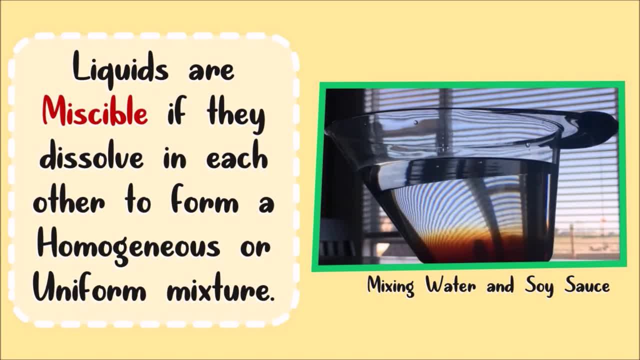 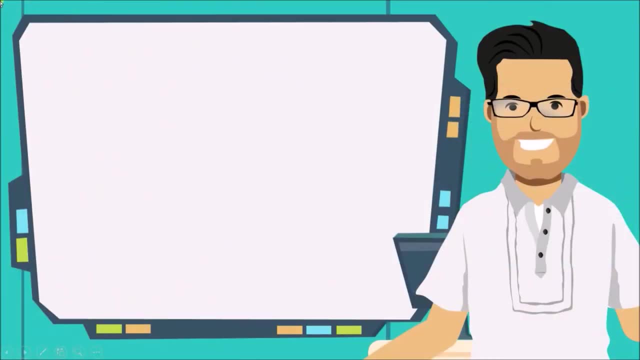 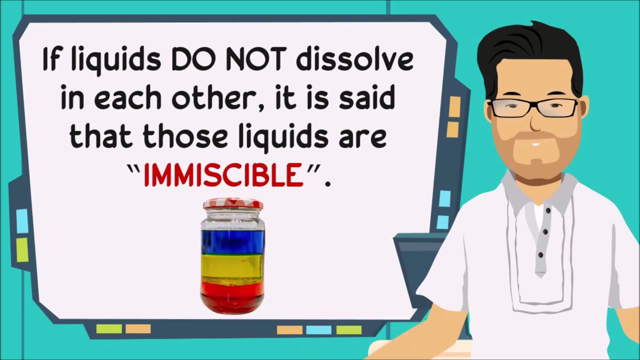 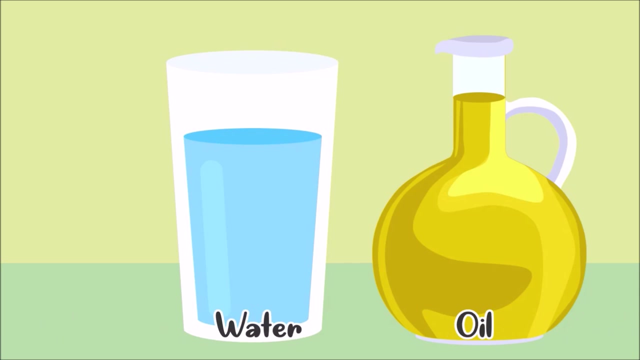 to form a homogeneous or uniform mixture. On the other hand, if liquids do not dissolve in each other, it is said that those liquids are immiscible. Have you ever tried mixing water and oil? What did you observe? That's right. 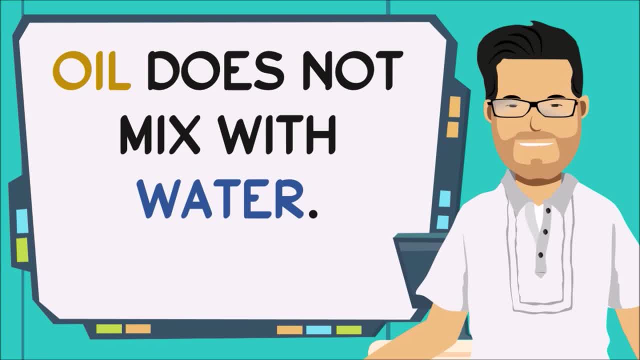 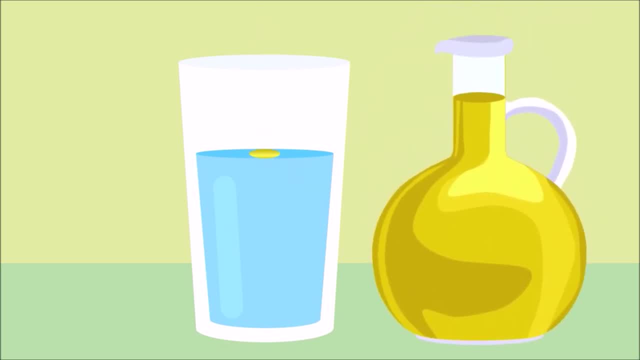 Oil does not mix with water. When a small amount of oil is mixed with water, the oil floats on top of water as little blobs, And when so much oil gets spilled on water, it forms a layer on top of the water. Therefore, 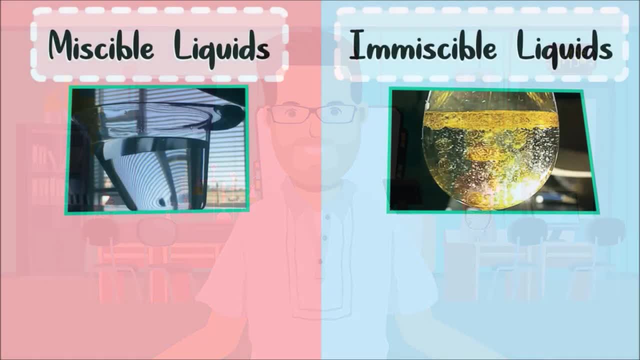 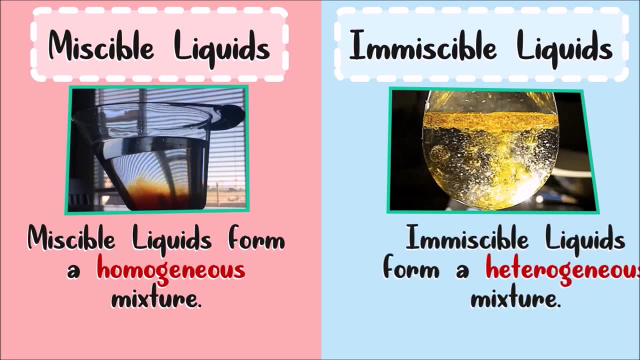 if we compare miscible and immiscible liquids, we will know that miscible liquids form a homogeneous mixture, while immiscible liquids does not, Because, like liquids, they are mixed with water. If we compare with an oil mixture, it is a heterogeneous mixture. 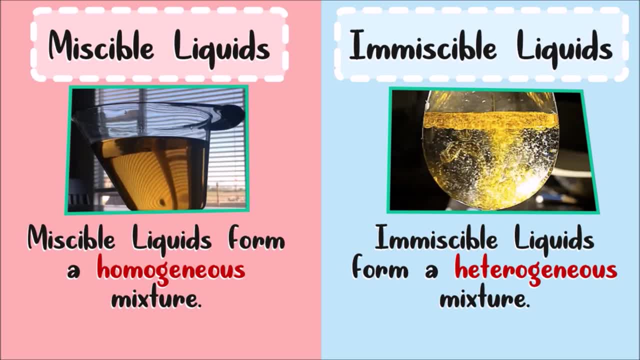 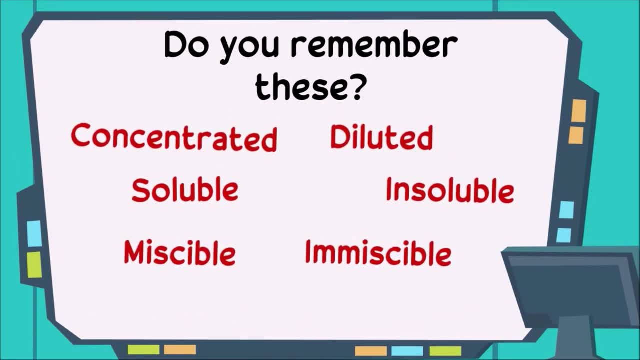 a mixture of water and oil. In a mixture of oil and water. it is a heterogeneous mixture. It is a heterogeneous mixture Like sulfide or glycine. it is a mixture of oil and water, Although it is a mixture of oil and water.